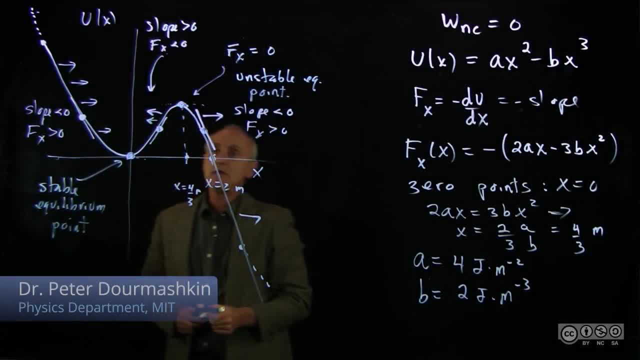 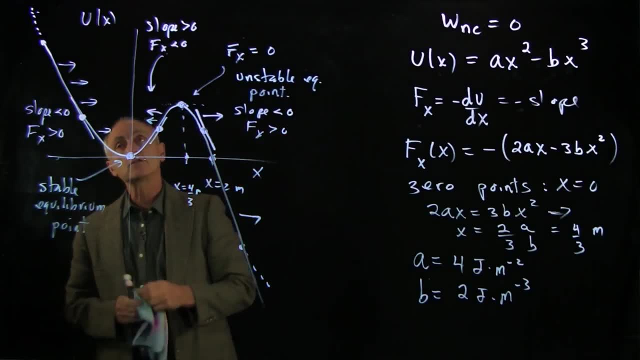 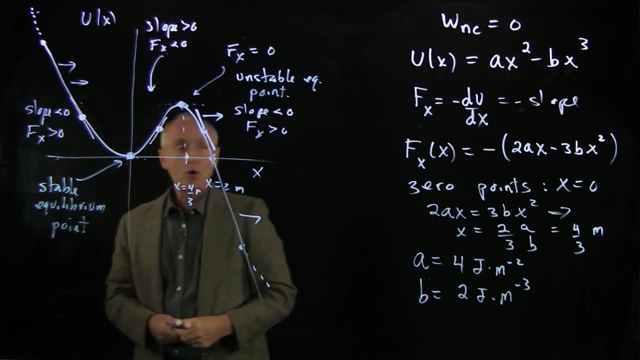 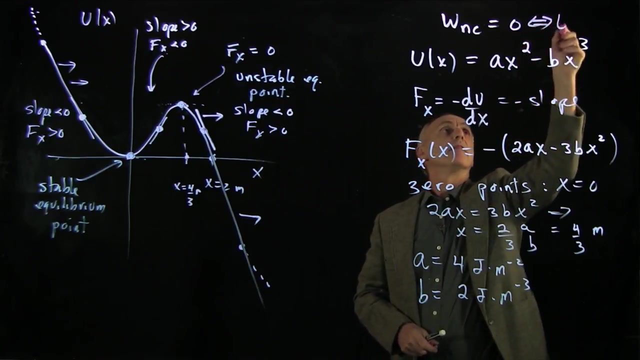 There's even a little bit more that we can learn about our energy diagram and I like to just clean this diagram up for a little bit of a second because I want to work in this area. Suppose our system, because the work non-conservative is zero, tells us that 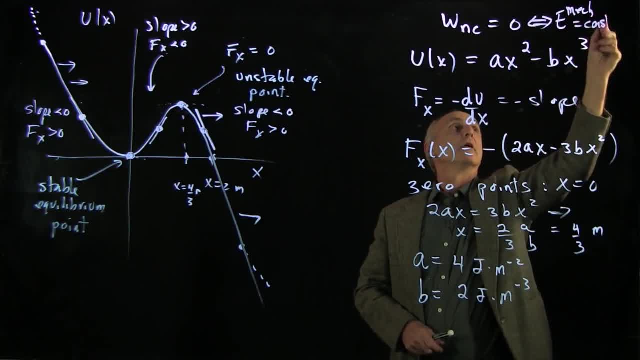 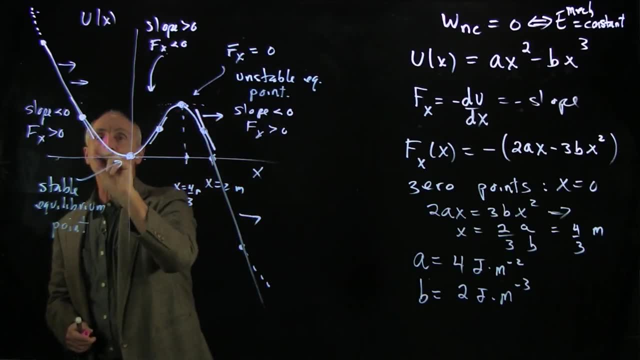 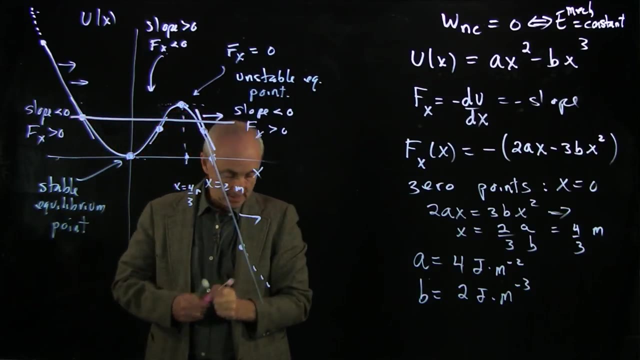 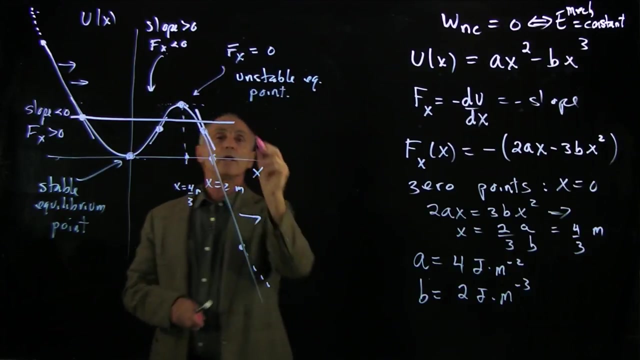 the mechanical energy is constant. Now we don't know how much mechanical energy our system is. That's a constant of the system. but let's just suppose that our mechanical energy is written like that. We'll just clean up a little, give ourselves a little space. 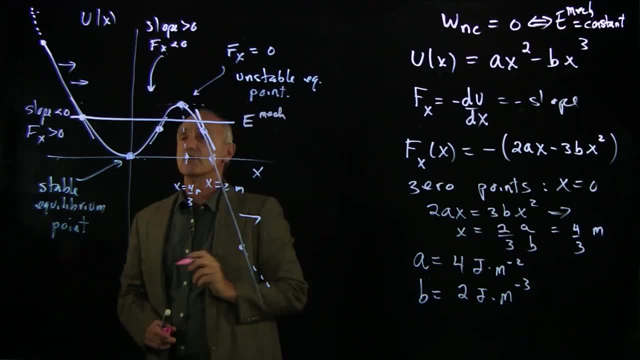 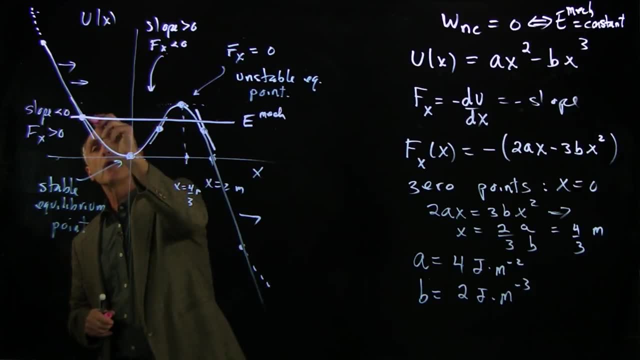 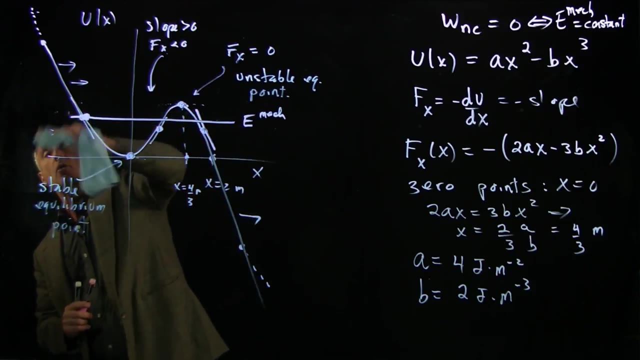 Here's the mechanical energy of the system, and that's a constant. Now we can talk about two more special points, a point over here, and at this point let's just think about what our mechanical energy tells us. This is a special point, but let's. 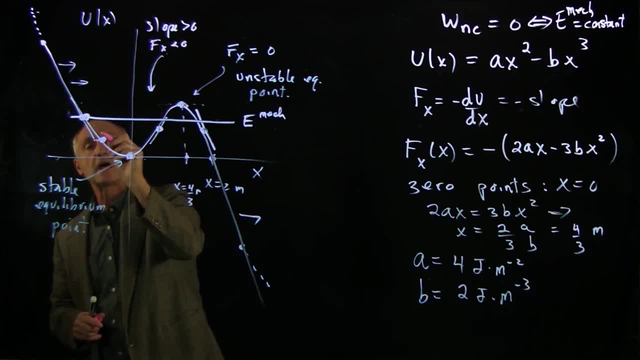 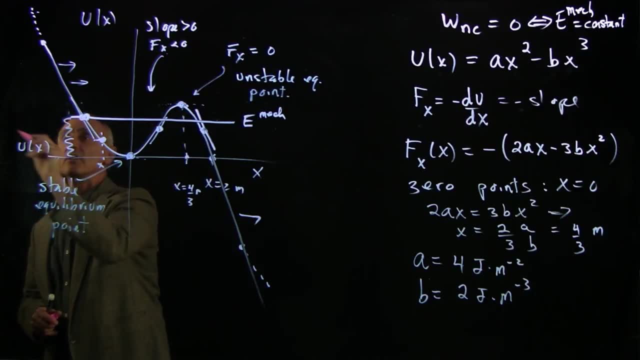 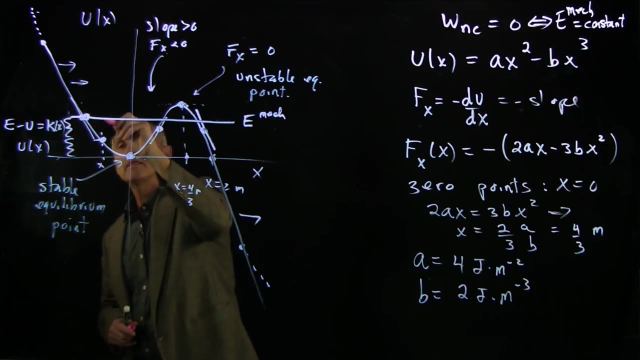 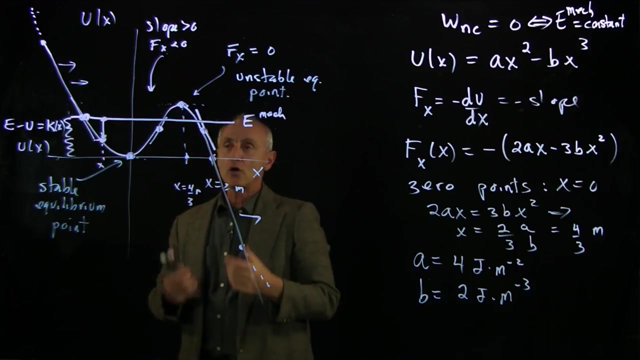 begin with one right here. If our particle is at this location, then this represents the potential energy, and the difference between the energy and the potential energy is the kinetic energy. So this here represents the kinetic energy. And now we can ask ourselves what. 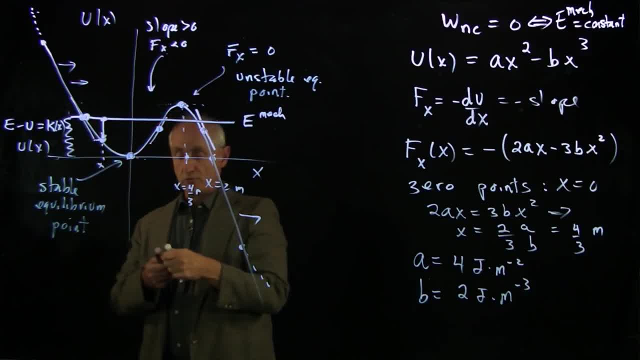 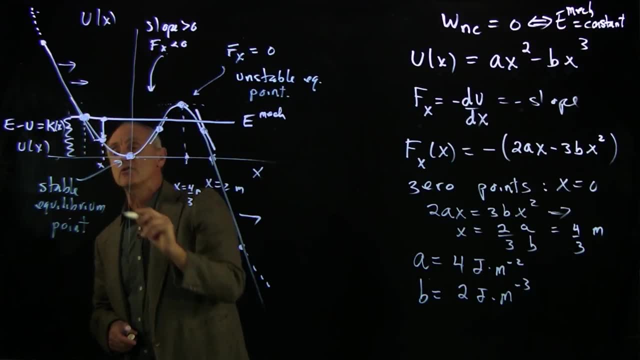 would happen to the energies as our particle is moving. So if we start right here, the kinetic energy is 0, because all the energy is potential And as a particle starts to move- let's say it has a little bit of energy- it starts to move in this direction. 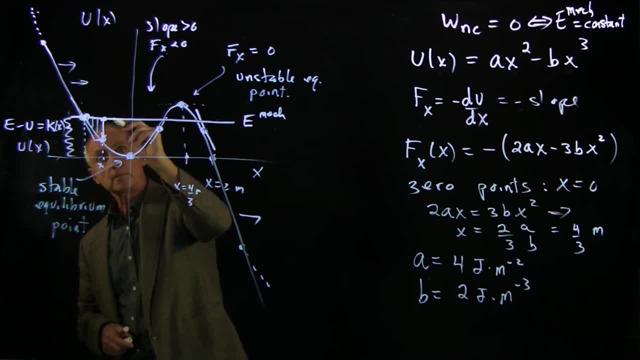 then the kinetic energy starts to increase until we get to this point where the kinetic energy is maximum, at the stable equilibrium point, where the force is 0. Now the kinetic energy decreases because, remember, it's now going against the force. This side the force was pointing in that direction. 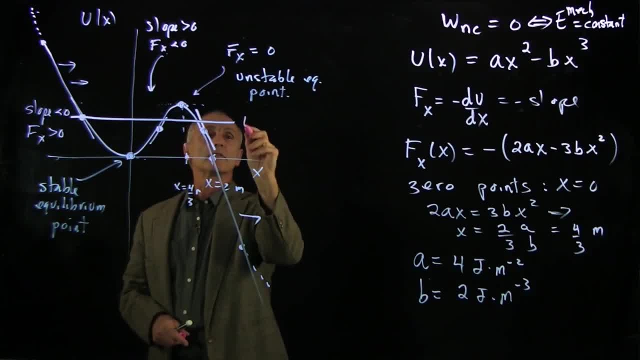 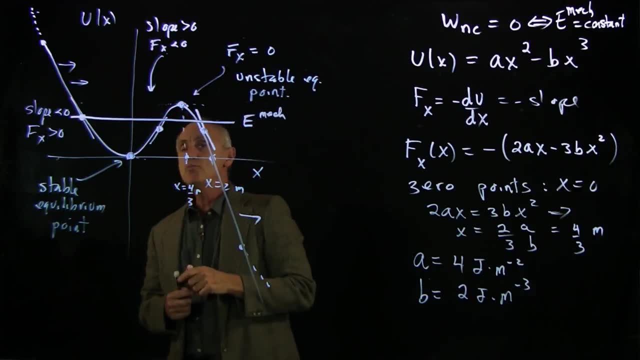 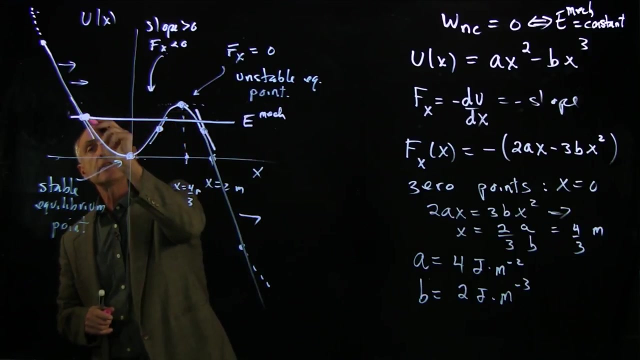 space. So here's the mechanical energy of the system, and that's a constant. And now we can talk about two more special points, A point over here, and at this point let's just think about what our mechanical energy tells us. This is a special point, but let's begin with one right here. If our particle 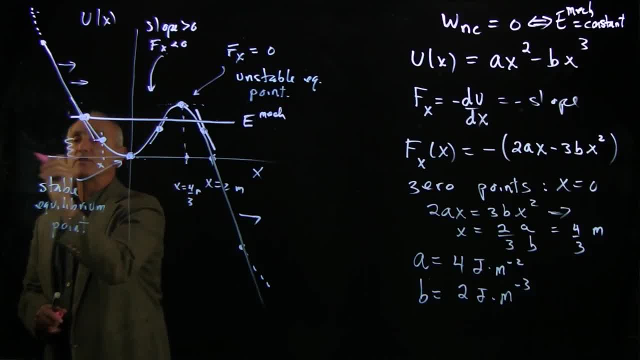 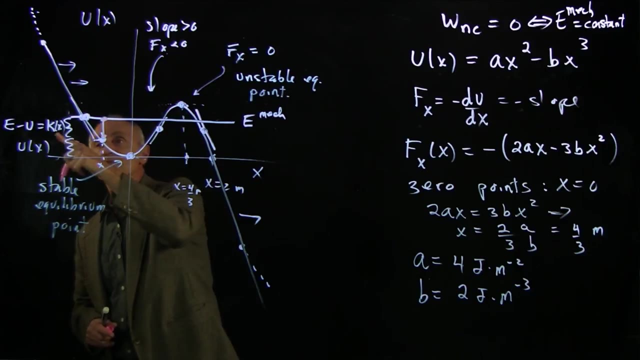 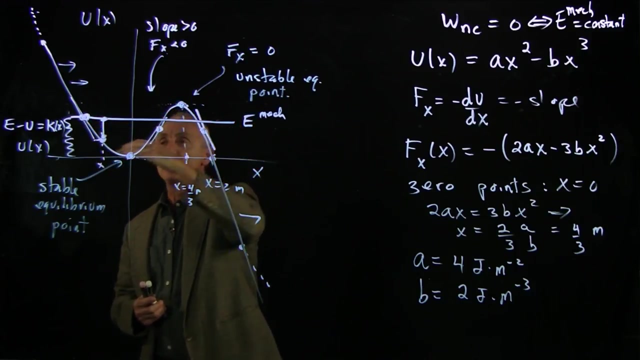 is at this location, then this represents the potential energy, and the difference between the energy and the potential energy is the kinetic energy. So this here represents the kinetic energy, And now we can ask ourselves what would happen to the energies as our particle is moving. 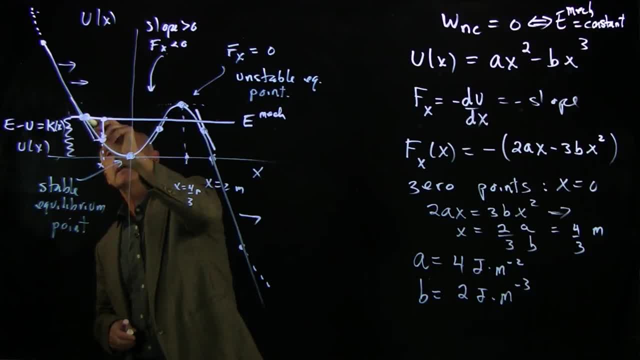 So if we start right here, the kinetic energy is 0, because all the energy is potential And as a particle starts to move- let's say it has a little bit of energy- it starts to move in this direction. then the kinetic energy starts to increase. 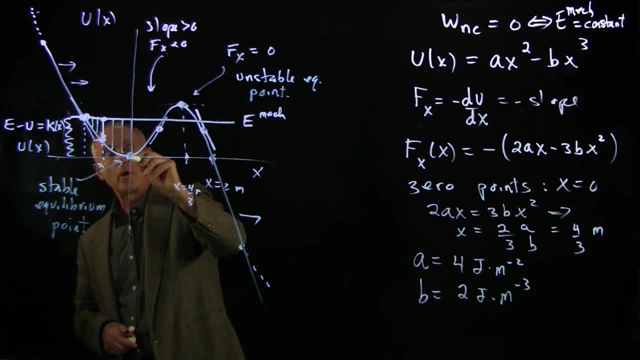 until we get to this point where the kinetic energy is maximum, at the stable equilibrium point, where the force is 0.. Now the kinetic energy decreases because- remember, it's now going against the force This side. the force was pointing in that direction here. 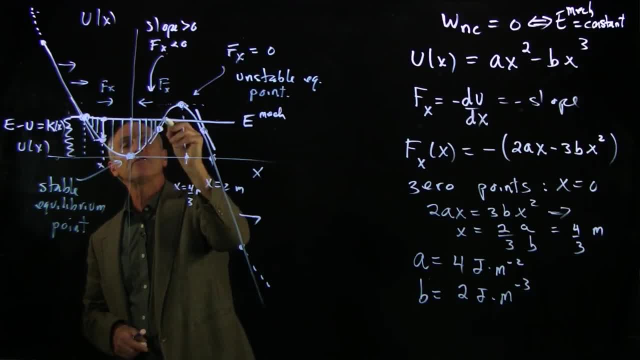 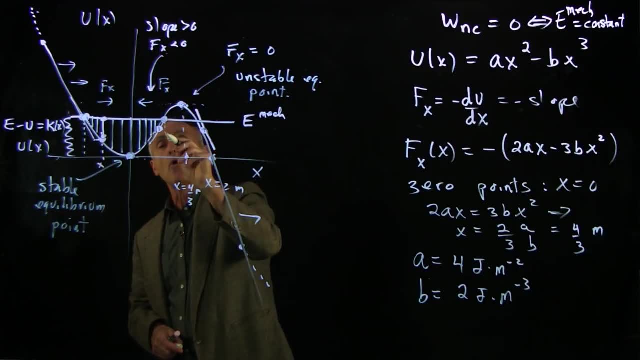 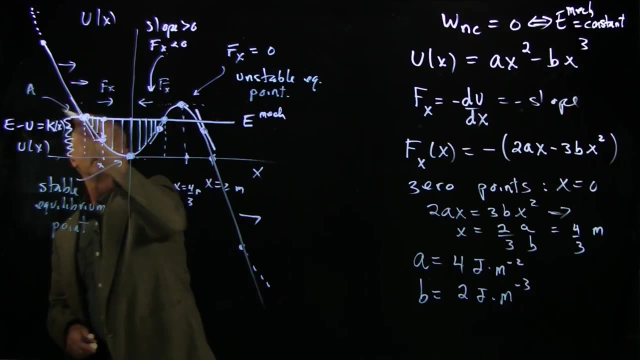 It was in the other direction, And until we finally get to this point where, again, the energy of the system is equal to all potential energy and so there is no kinetic energy. So I'll call this point a And I'll refer to this point over here. 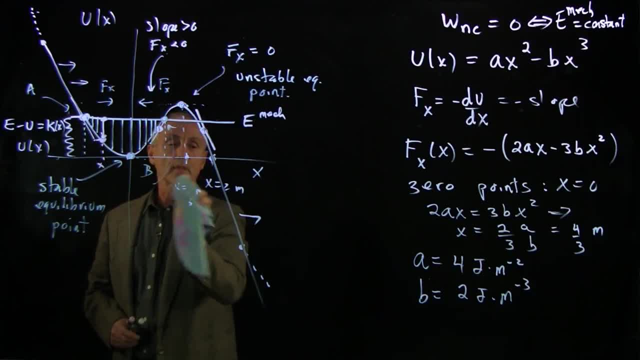 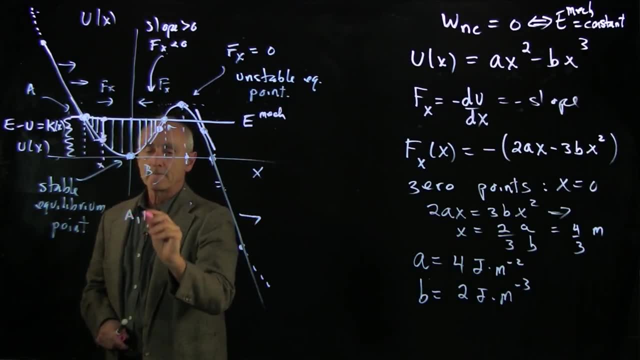 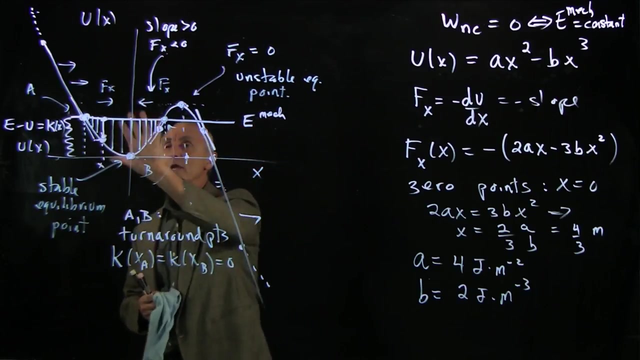 Diagram is getting a little crowded as b, And those points a and b are what we call the turnaround points, And they represent the places where the kinetic energy at xa is equal to the kinetic energy at xb, which is 0.. Now the last thing that we like. there's a lot of information. 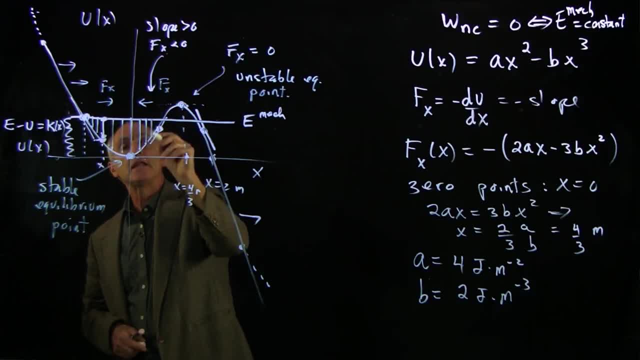 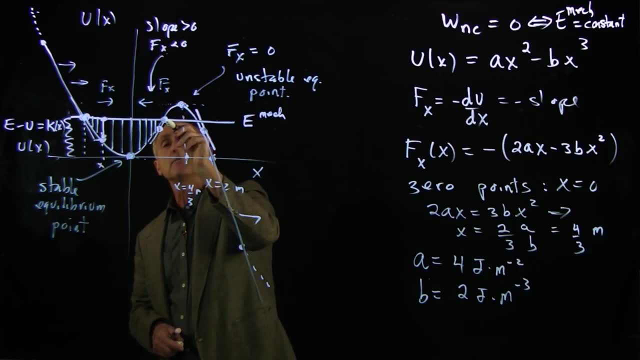 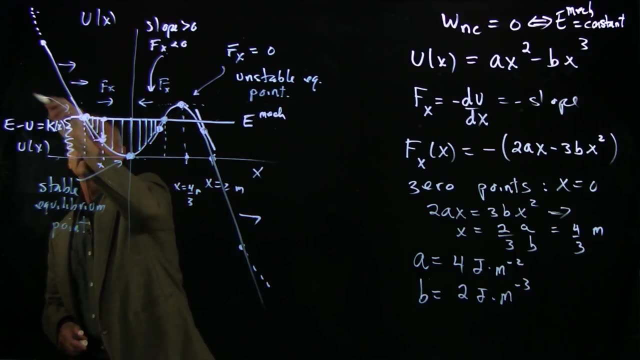 here It was in the other direction, And until we finally get to this point where, again, the energy of the system is equal to all potential energy and so there is no kinetic energy. So I'll call this point a And I'll refer to this point over here. 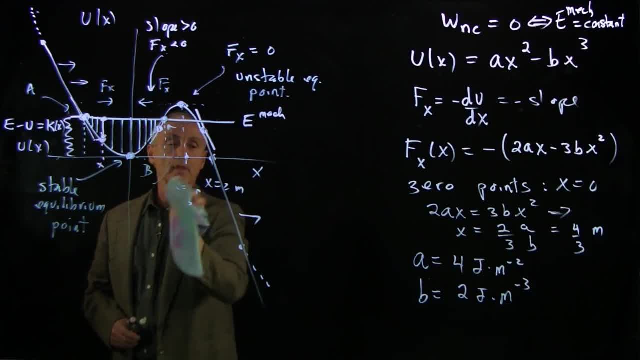 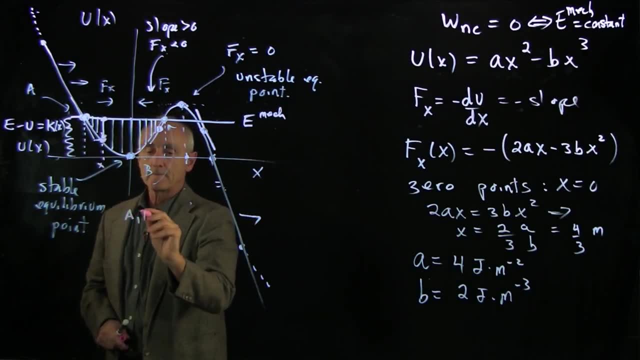 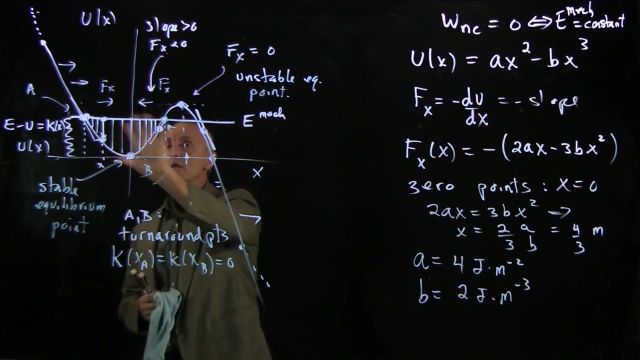 Diagram is getting a little crowded as b, And those points a and b are what we call the turnaround points, And they represent the places where the kinetic energy at xa is equal to the kinetic energy at xb, which is 0.. Now the last thing that we like. there's a lot of information. 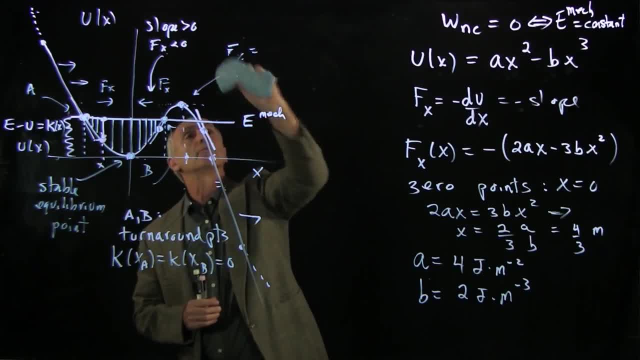 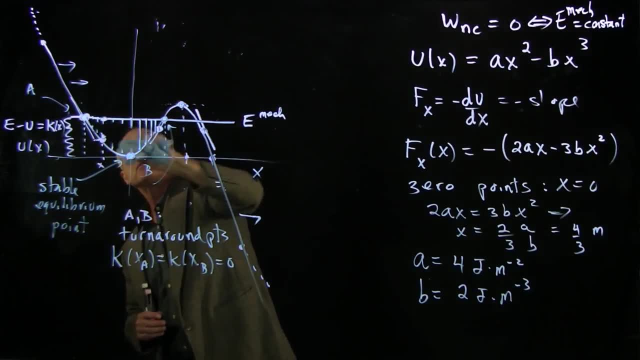 as you can see contained in these energy diagrams. And the last bit of information that we'd like to ask ourselves is what would happen if, instead of confining our system to this area, we increased our mechanical energy? so we're up here And let's just follow qualitatively. 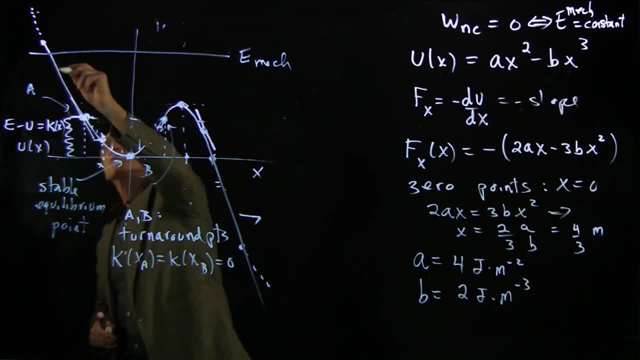 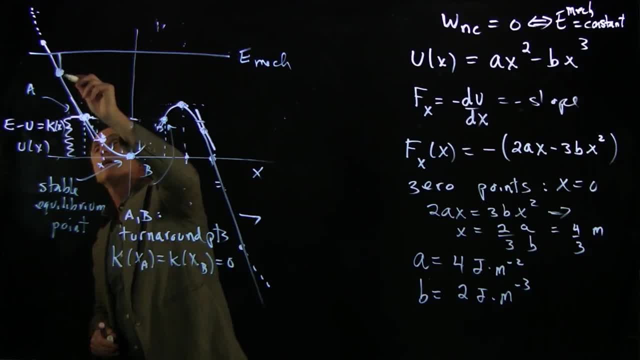 And we're up here Over here with a little bit of kinetic energy and potential energy And if the particle starts off with the velocity in the positive x direction, then it's going to move in this direction And you can see the kinetic energy is increasing. 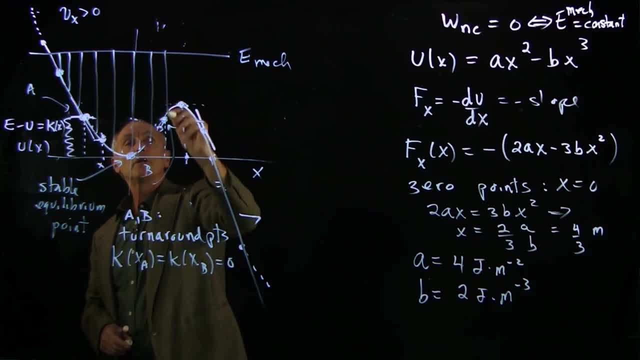 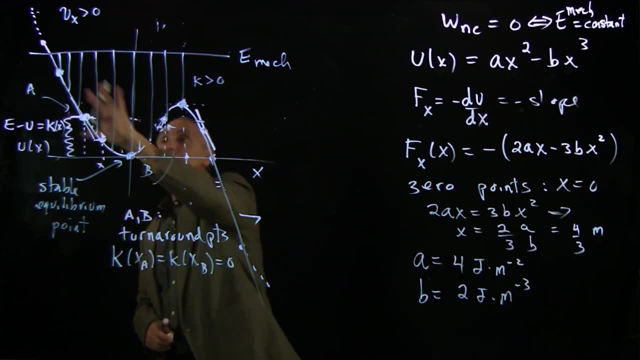 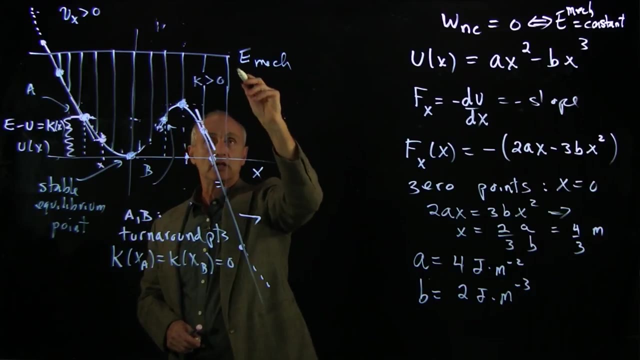 Here we have a maximum amount of kinetic energy, But notice that over here the particle still has some positive kinetic energy, And so it can get Over this hill, And when it gets to the other side the force was in the positive direction. 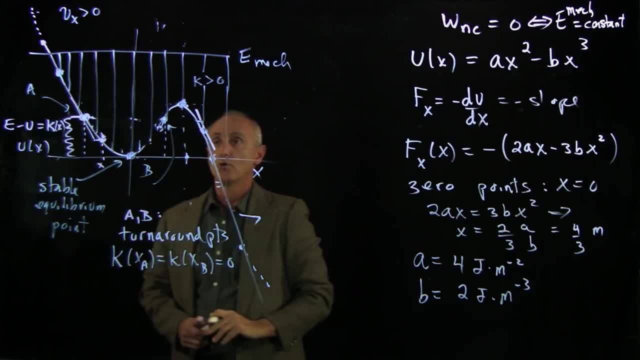 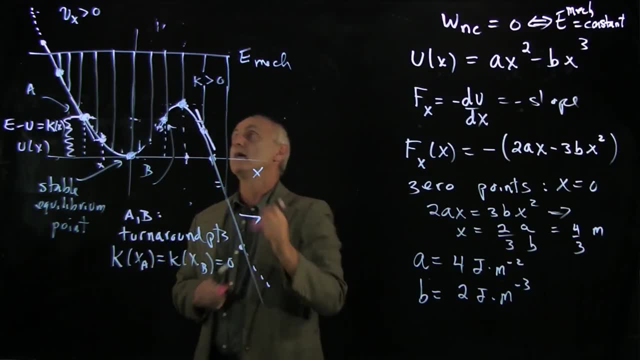 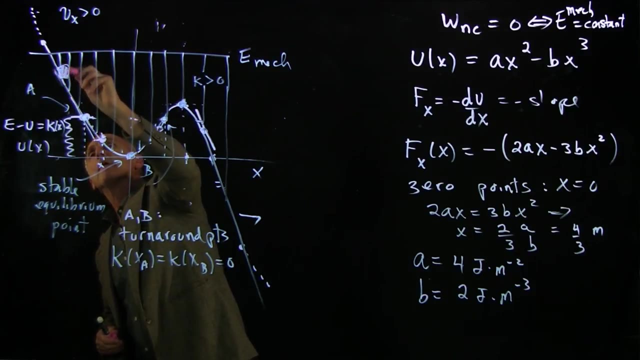 it increases its kinetic energy And it goes off to what we're referring to as infinity. So one analogy that people like to make is to understand the motion. Think of a marble that's rolling down a hill, And this is just a metaphor for this potential energy function.